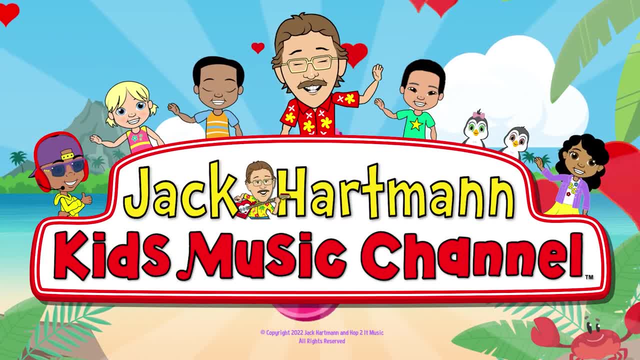 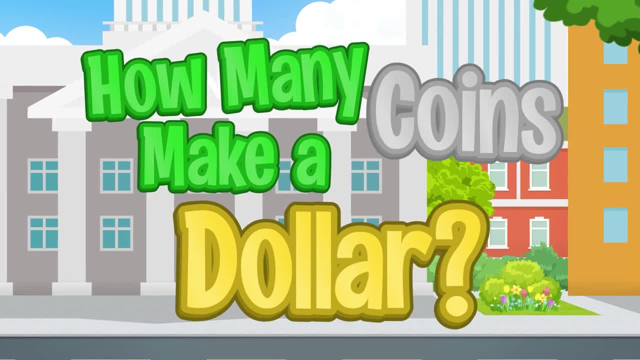 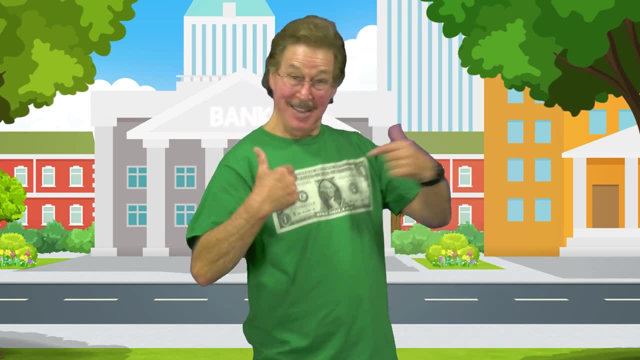 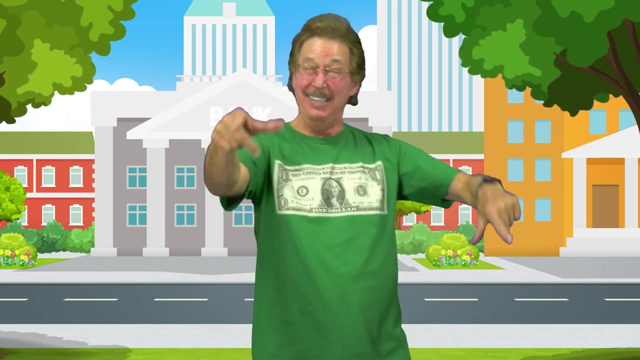 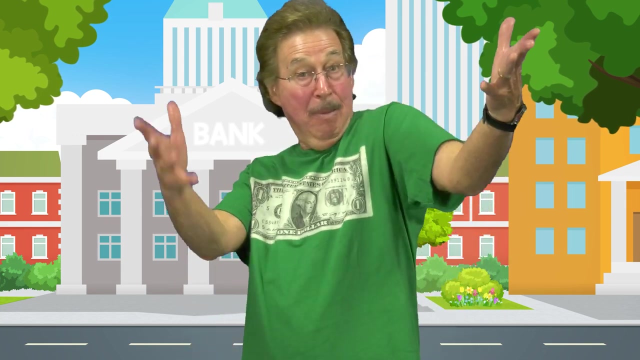 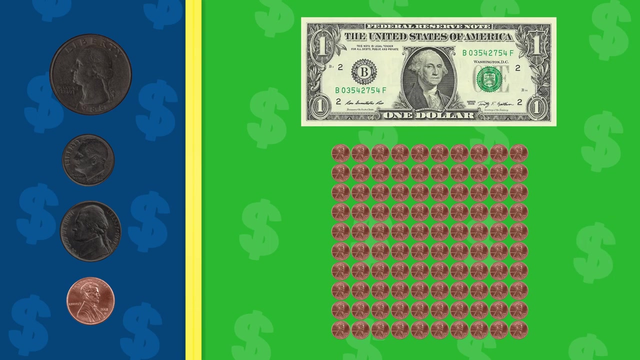 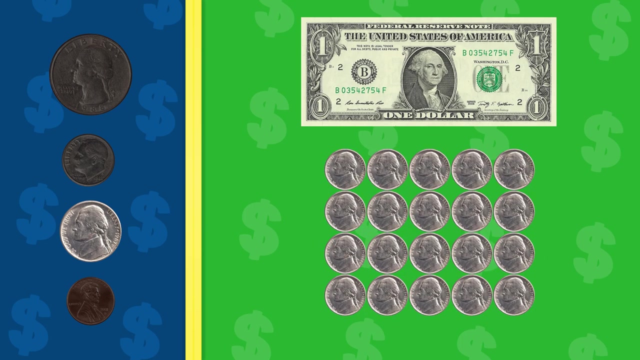 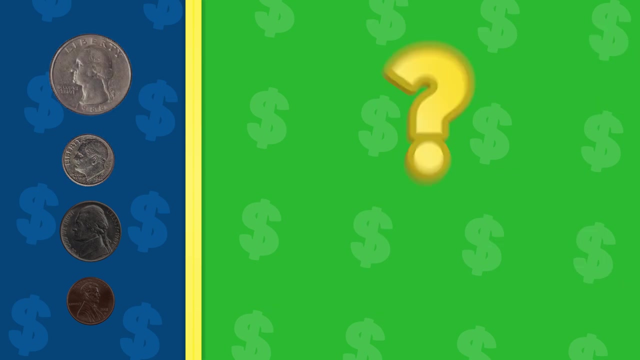 Jack Cartman. Kids in the Kitchen Say how many coins, twice How many pennies, make a dollar? One hundred, one hundred. How many nickels make a dollar? Twenty, twenty. How many dimes make a dollar? Ten, ten. How many quarters make a dollar? 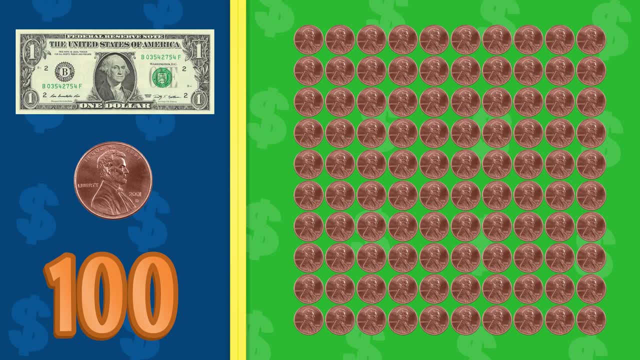 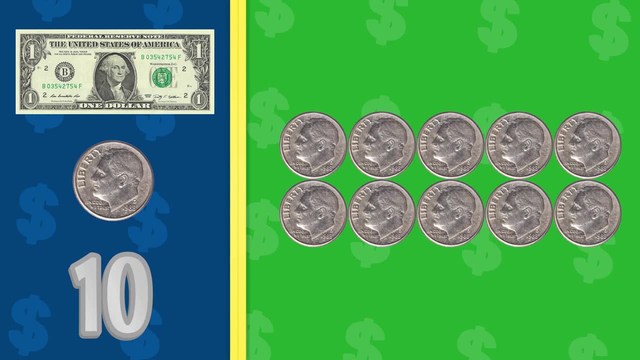 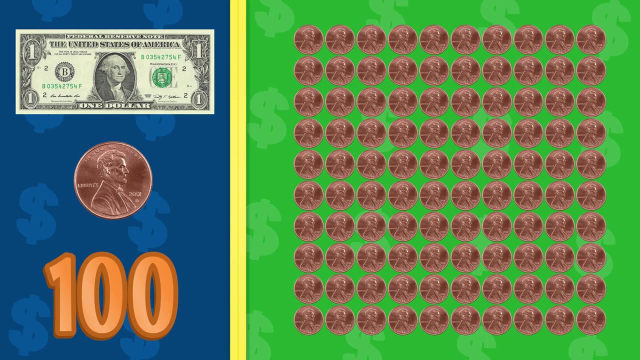 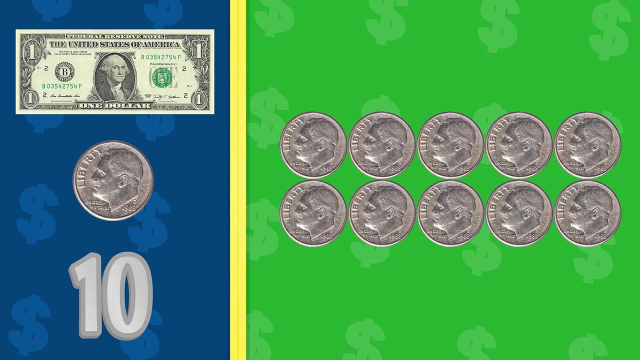 Four, four. One hundred pennies make a dollar. Twenty nickels make a dollar. Ten dimes make a dollar. Four quarters make a dollar. Now you sing it: One hundred pennies make a dollar. Twenty nickels make a dollar. Ten dimes make a dollar. Four quarters make a dollar. 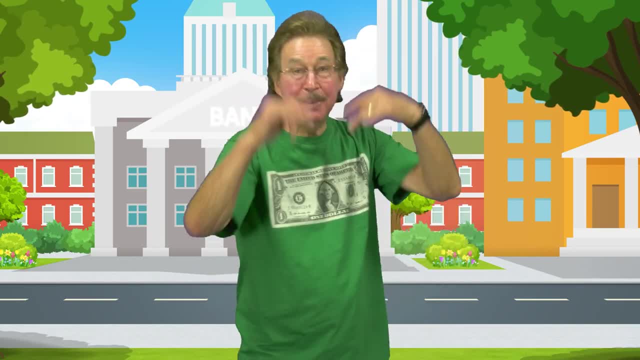 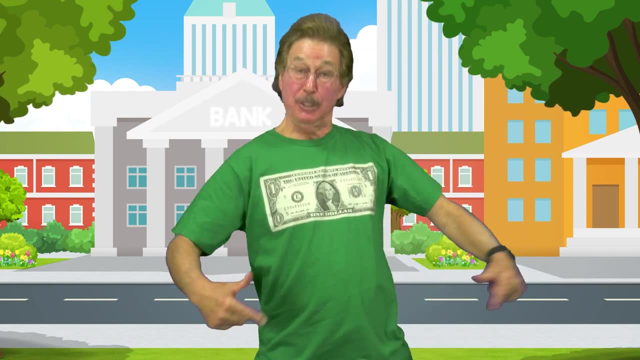 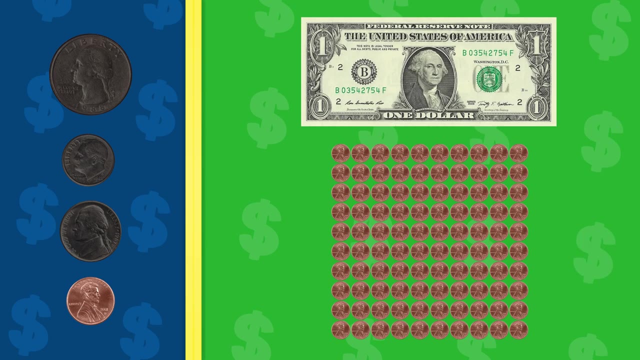 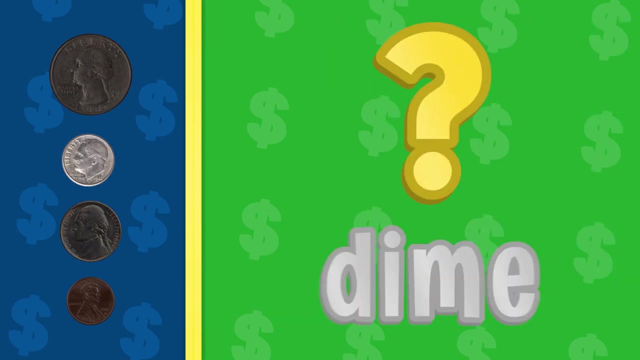 Count, count How many coins. how many coins make a dollar? Count, count How many coins. how many coins make a dollar. How many pennies make a dollar? One hundred, one hundred? How many nickels make a dollar Twenty twenty? 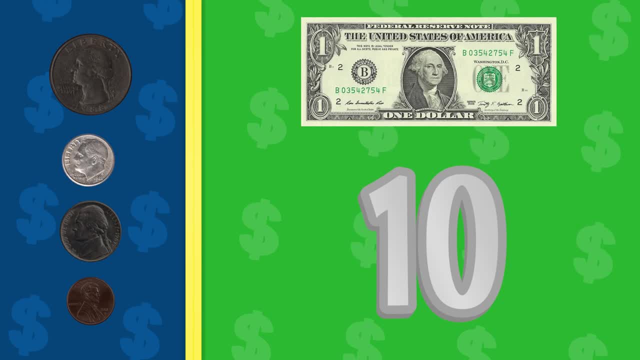 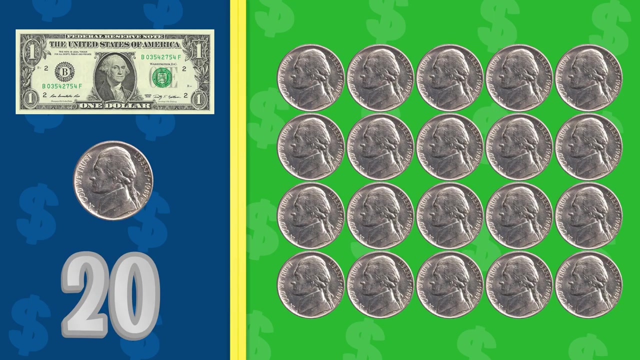 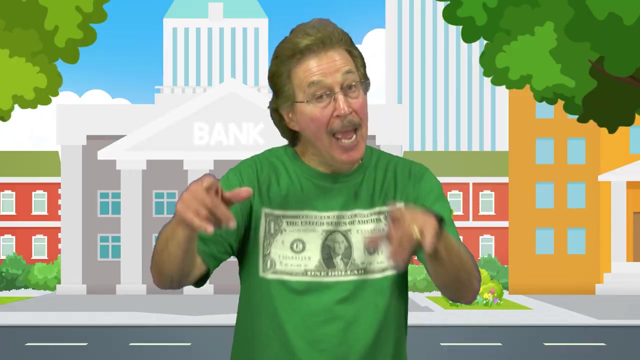 How many dimes make a dollar? Ten, ten, How many quarters make a dollar? Four, four, One hundred pennies make a dollar. Twenty nickels make a dollar. Ten dimes make a dollar. Four quarters make a dollar. Now you sing it: One hundred pennies make a dollar.